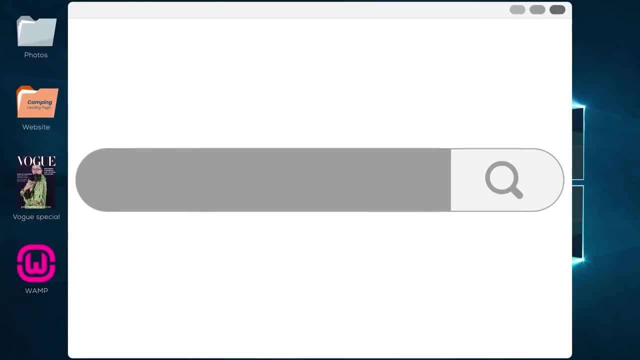 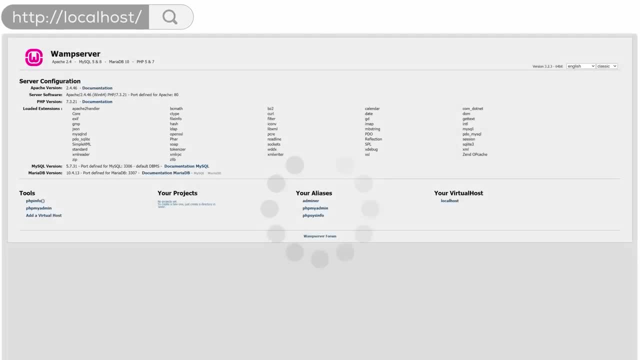 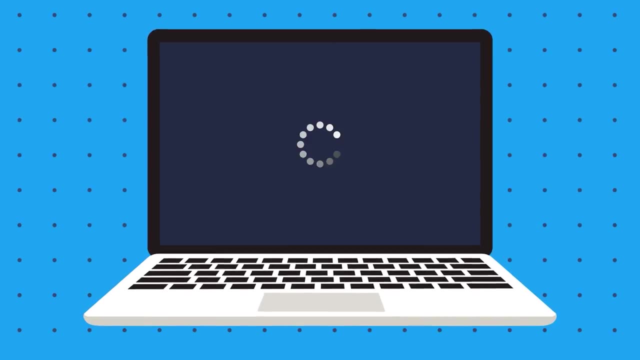 will be updated automatically. To test that, just type in http//localhost//. if you see this window, that means that everything is a-okay. my dudes, If not, try running the app again or restarting your PC. The good old fix it all hack. For this example, let's set up a WordPress website, So click. 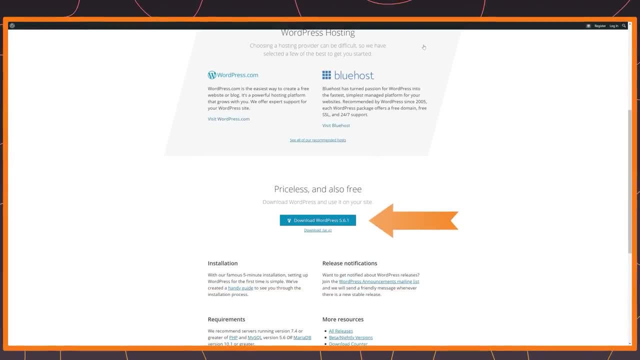 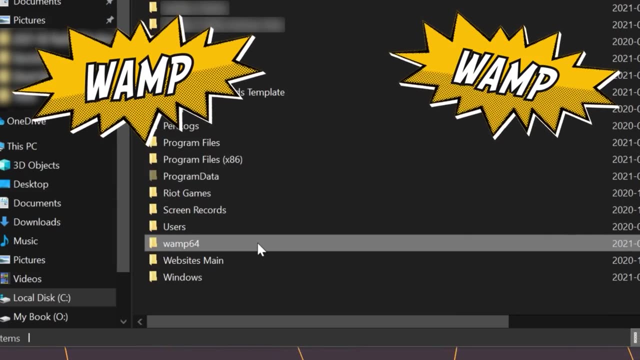 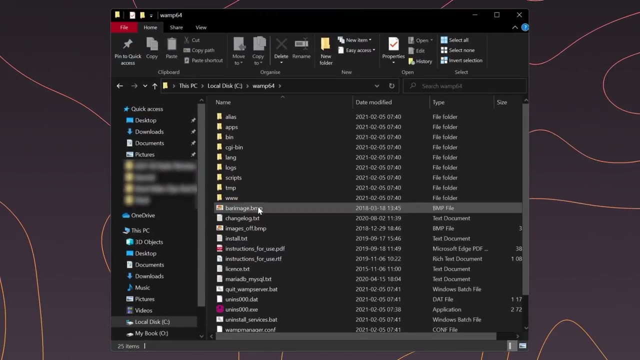 the link in the description, or just go to wordpressorg and download it to your PC Drive and find WAMP 64 or WAMP 32, depending on your install, And yes, I will say WAMP every single time because I find it super fun. You'll see a folder named www. Enter it and create a. 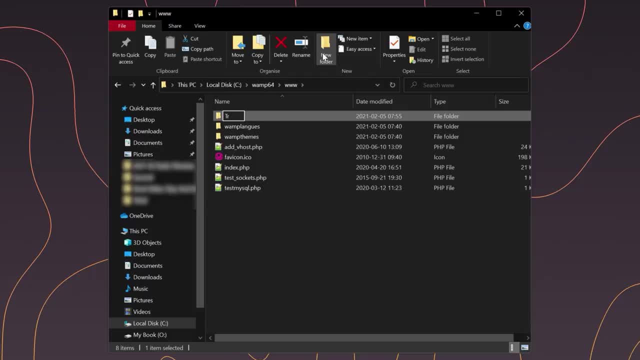 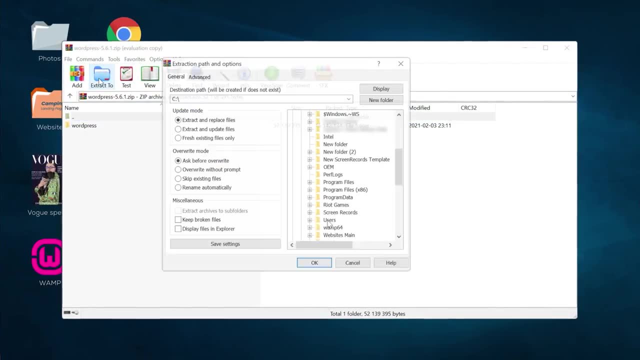 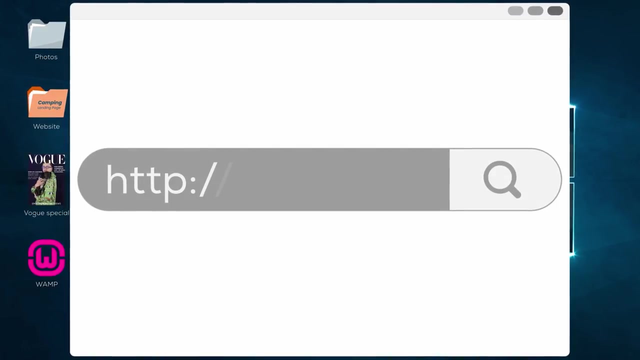 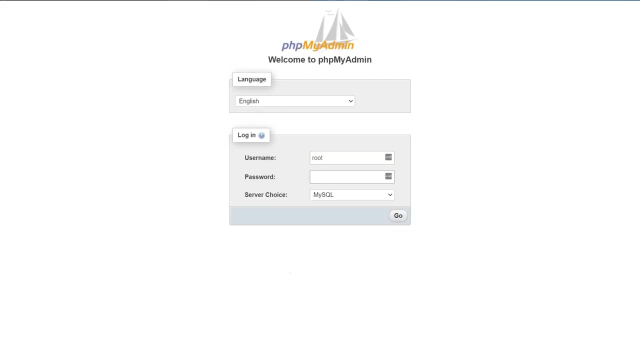 folder there. Name it whatever you want your site to be. Just don't leave any spaces here. Now open the WordPress RAR and extract it into the newly created website folder. Once that's done, just type in http//localhost once more. Click phpmyadmin at the bottom of this page. By default. 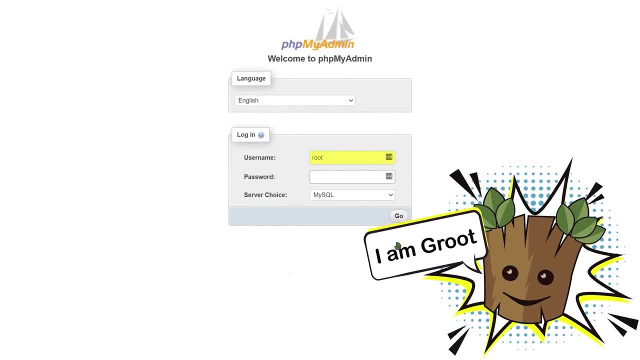 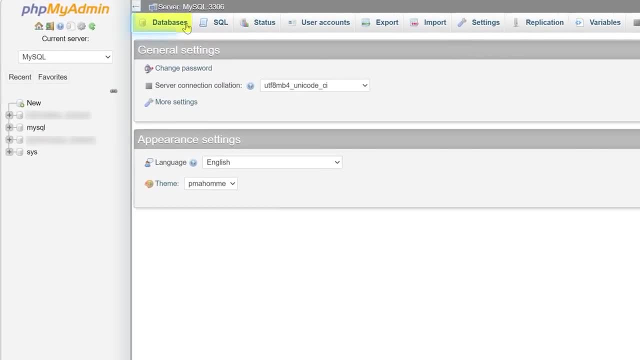 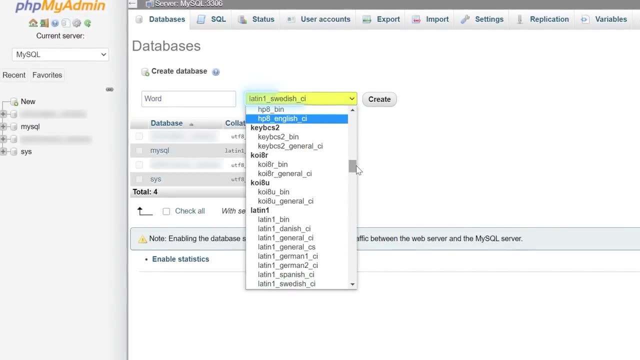 the admin username to your php will be root. Type it in and leave the password field completely empty. Then click go. Once you're there, click databases, type in the new database name, something like word as in WordPress- and select collation in the second selection. 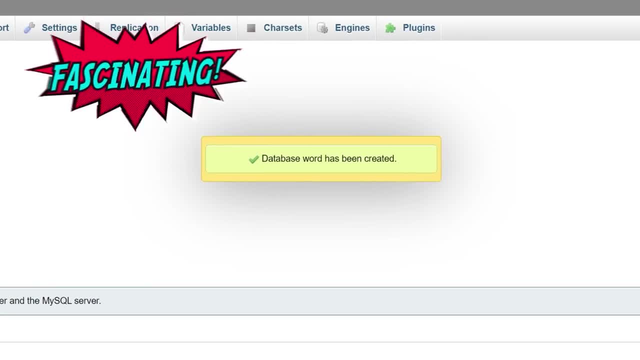 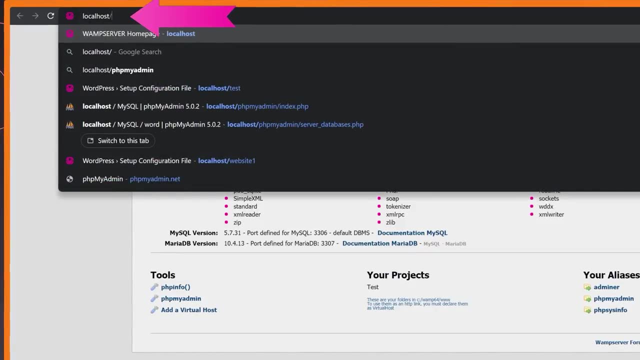 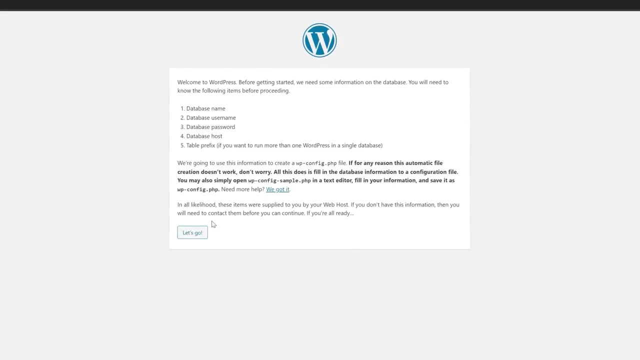 Finally, create the database by clicking create Fascinating Type in localhost and write the name of the folder you created in the www folder. In my case it would be test. You'll see the good old WordPress install screen. Select your language, go through the setup steps and enter the database name you just created. 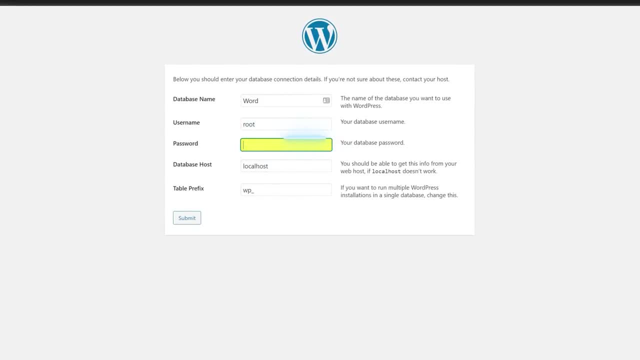 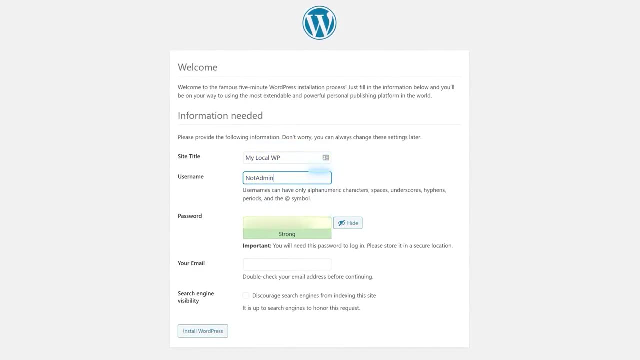 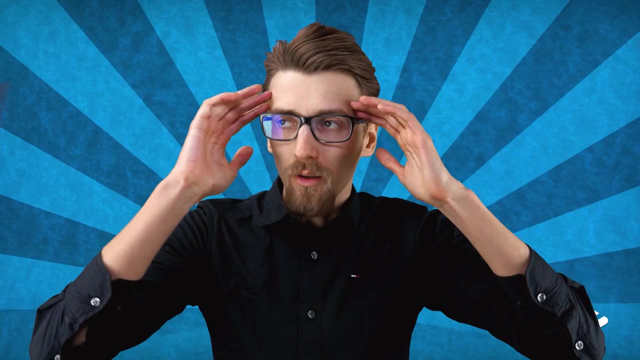 For username, add root and leave the password field completely empty. Next, add in all of the regular WordPress site information like site name, admin login and password. Let the installation do its thing and your local website will be live, And you can go nuts with this WordPress website. You can test different designs. 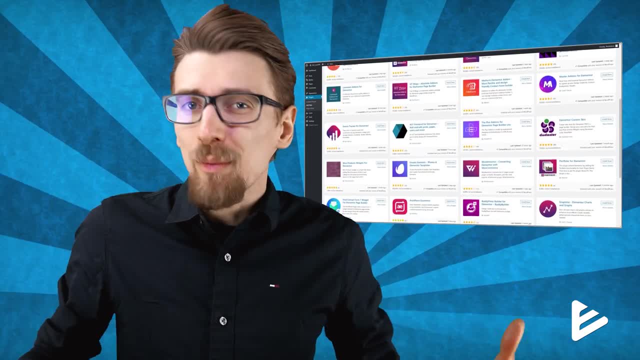 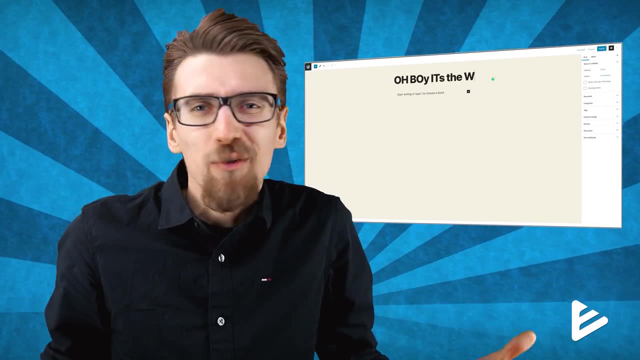 you can test plugins, you can test your code, you can see how different elements interact with each other- Basically, do anything, because it exists only on your computer, So there's nothing to break really. So here's the WordPress website Now you might want. 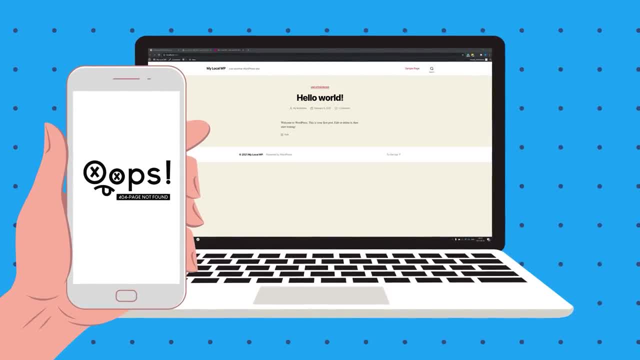 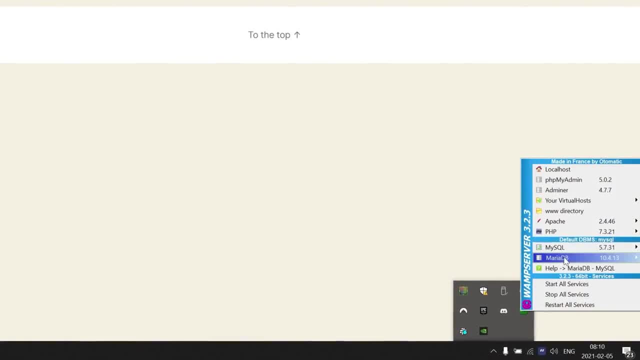 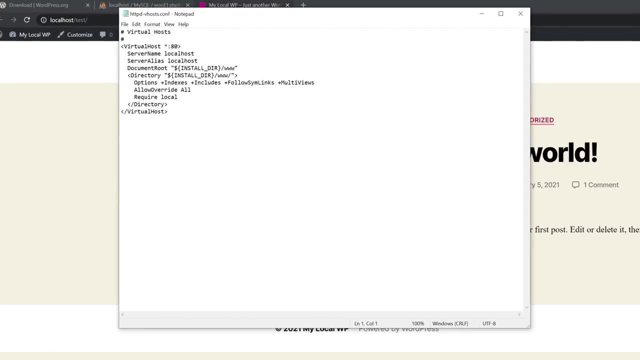 your site from different devices in your network, not just your local PC. To do so, go to the icon, click the left mouse button, select Apache and click httpd vhostconf. It will open a text editor app, probably notepad, so just. 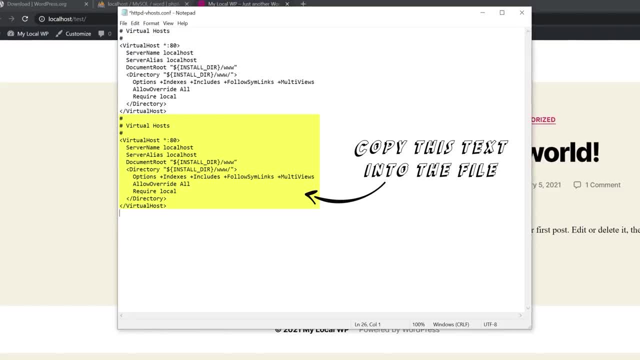 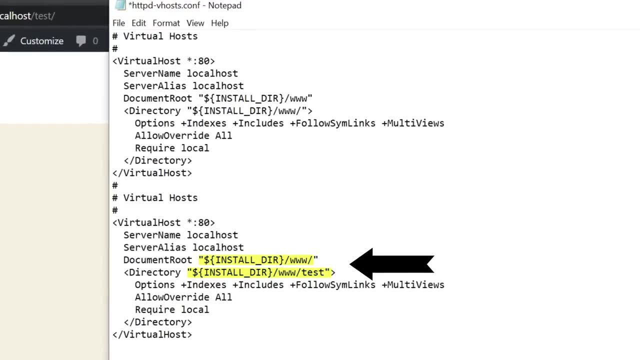 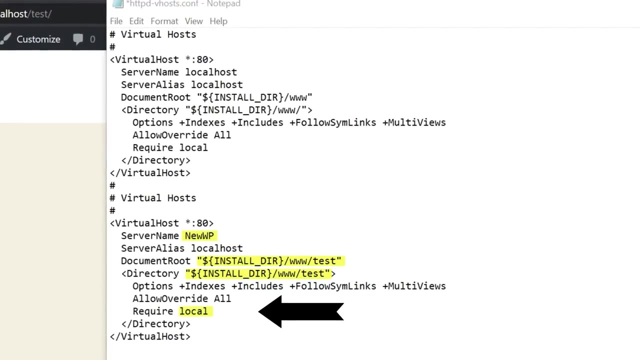 copy this text into the file. I'll leave it in the description or a comment down below The install DIR to where your www folder is located and change the server name if you have a few different projects. Change required to either allow the IP addresses or just all granted for anyone in your local network to have. 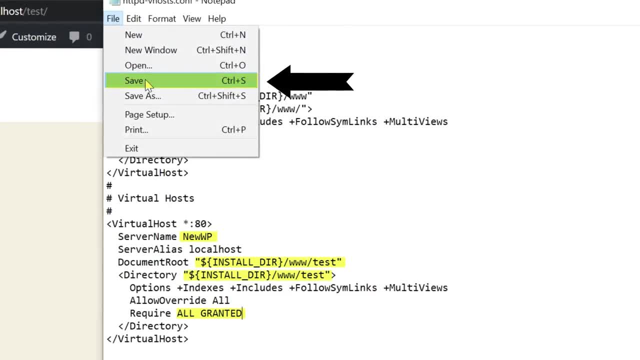 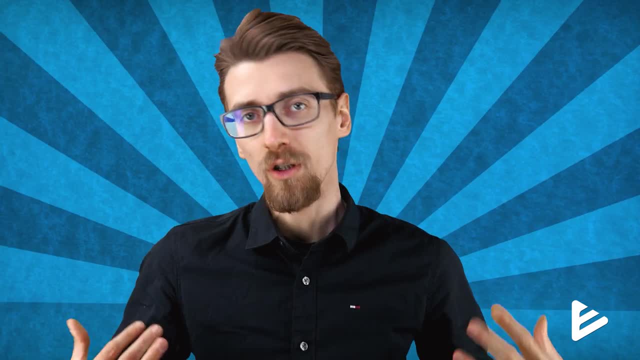 access And, of course, don't forget to save your file. But even after all of that, your website is still just a local website, meaning it's available only to your device and the local network around you. If you want to put this website on the internet, you'll need to open up some. 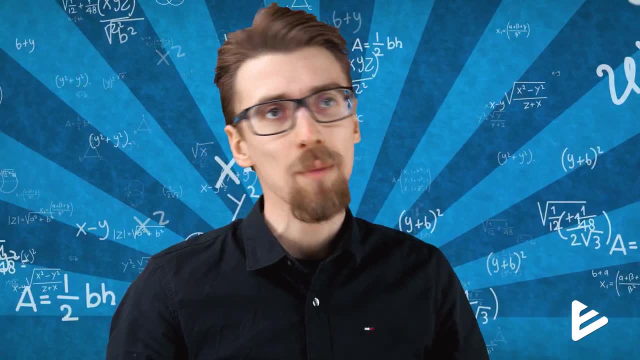 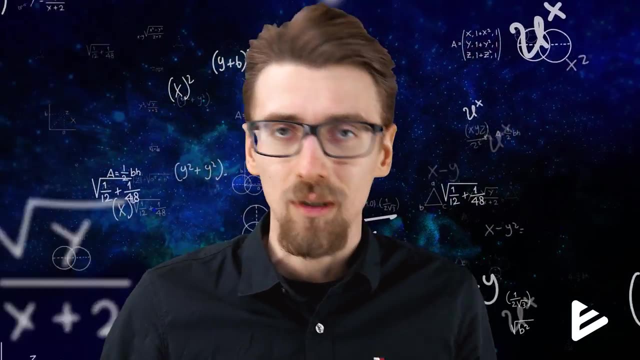 ports, open up some connections and point your IP address to the website or a domain name, and people will use the IP address or domain name to access the website. It sounds complicated, but it really isn't. well, maybe it kind of is. Don't worry, I'll just show you how to do it. 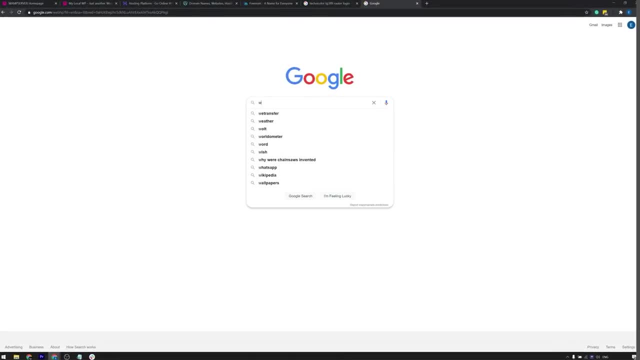 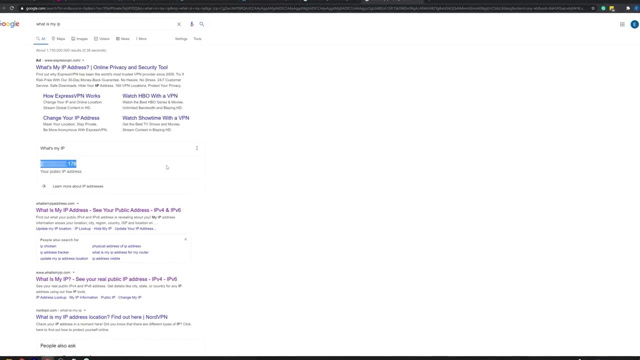 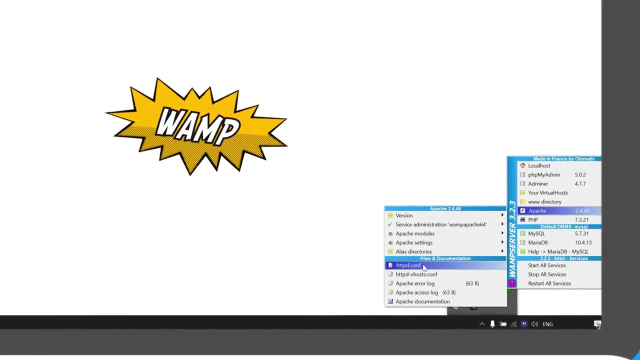 To find out your IP address, just go to Google and type in what is my IP, or click the link in the description down below. It will give you your IP address that you need to connect to Now click your WAMP icon and select Apache From the drop-down menu select. 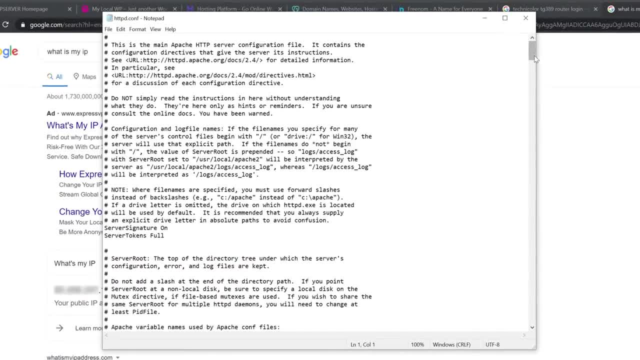 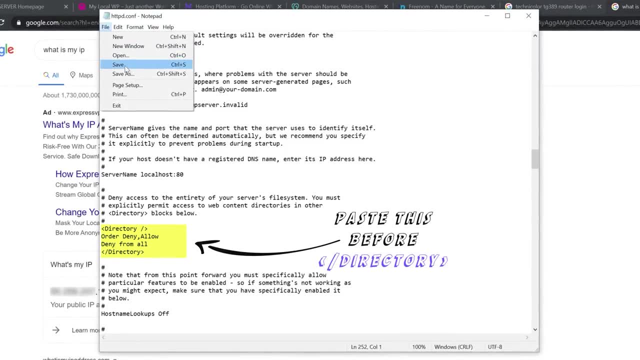 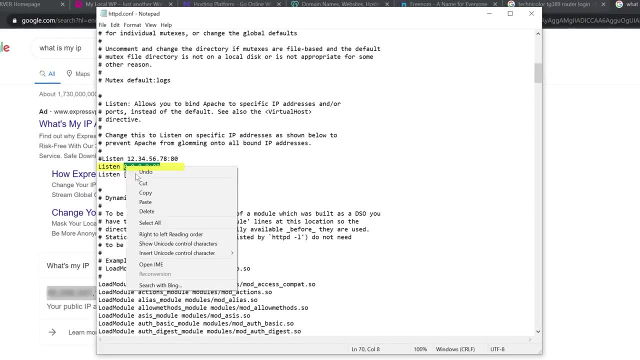 httpdconf and it will open a text editor. Find directory and change the value in there. Paste it before the directory tag closes. Then we need to find listen000080 and change the numeric value to your IP address. Then find a server name and add your IP here again. 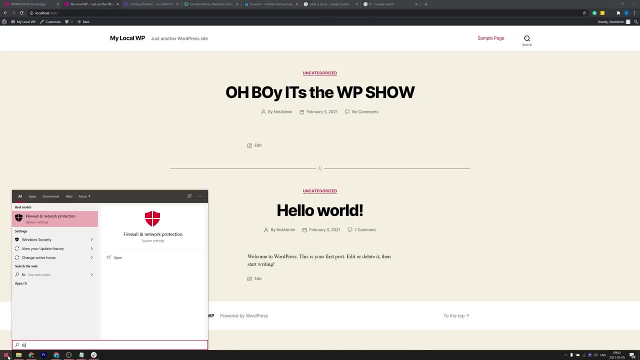 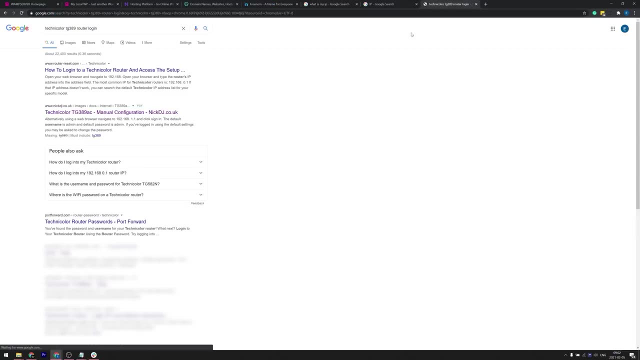 Now you will need to turn off your firewall or configure it in a way so it would allow incoming connections. For this example, I'll just turn it off. Next, you have to access your router. Look up its model. then you can find your modem administrator IP by just googling the router's name together with the word. 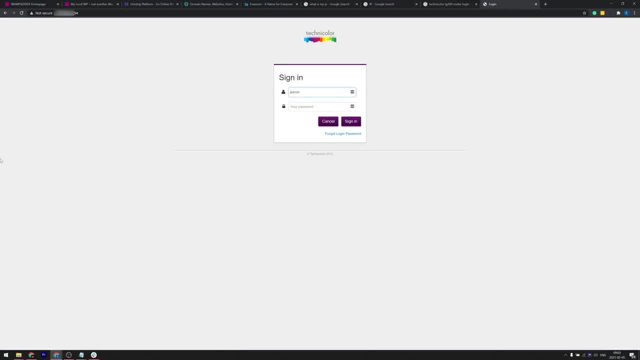 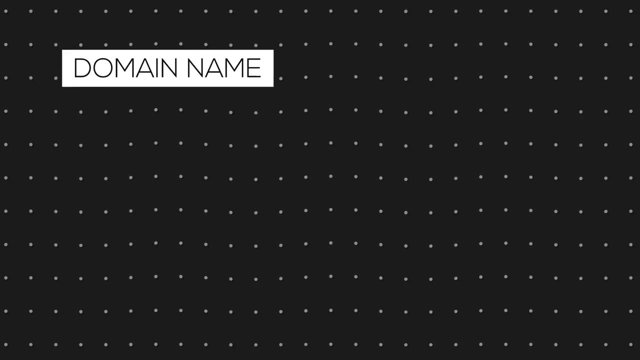 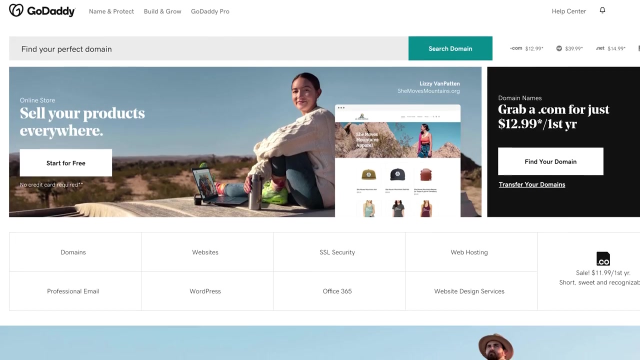 login Once you access the login page. most routers have either a simple root name and password, or it might be on the back of your router. Now, to link a domain name to your IP address, you will first have to have a domain name. If you don't already have one, just grab one from GoDaddy or 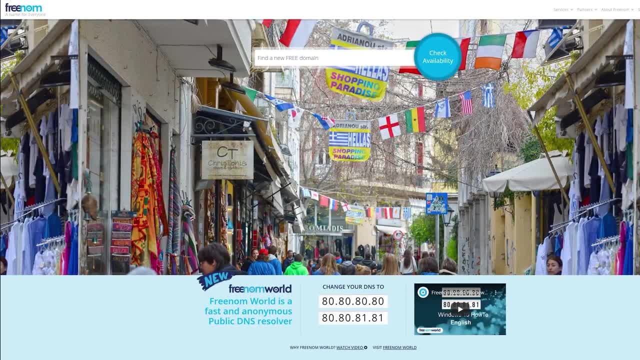 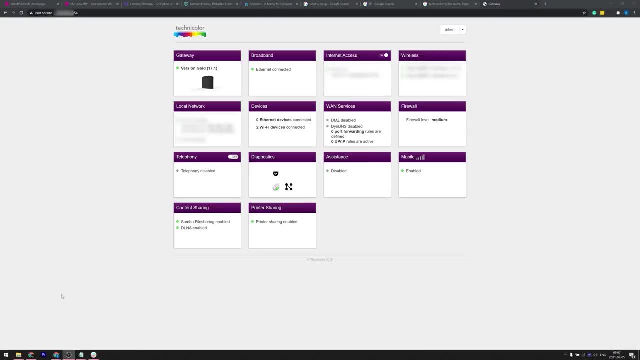 Hostinger or a free one from Freenom. I think there's no need for me to explain how to get a website name registered. Once you have your name ready and you're in your router's control panel, go to the port forwarding section and create a. 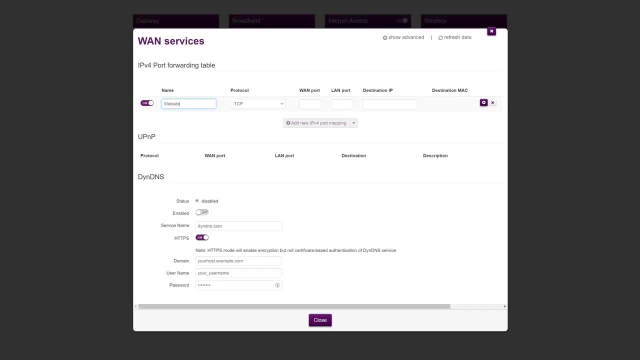 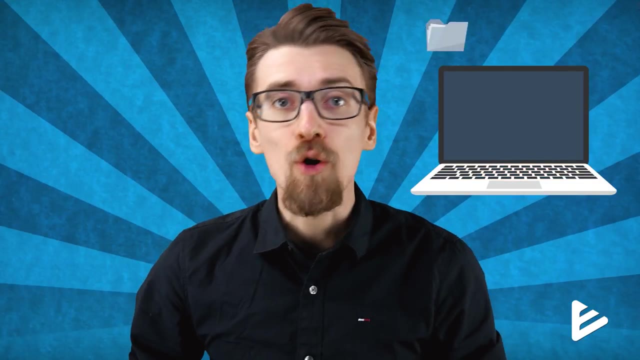 rule to forward port 80.. Also, make sure that your router allows incoming connections through port 80.. Once that's done, restart your WAMP and type in your IP address on another PC. It should link to your new website. What we basically did is store a bunch of 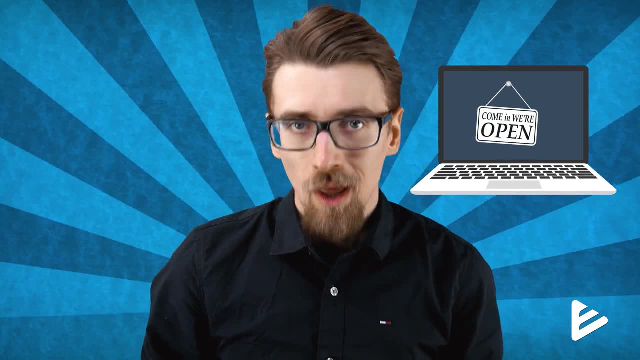 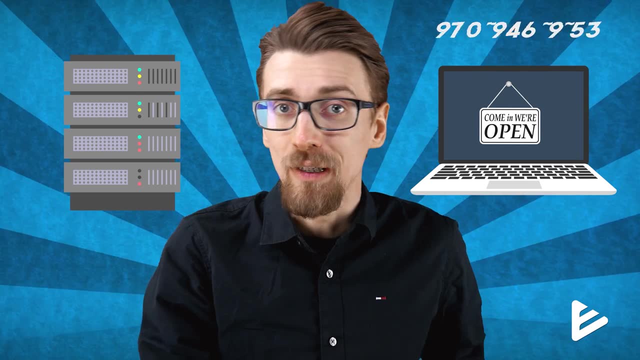 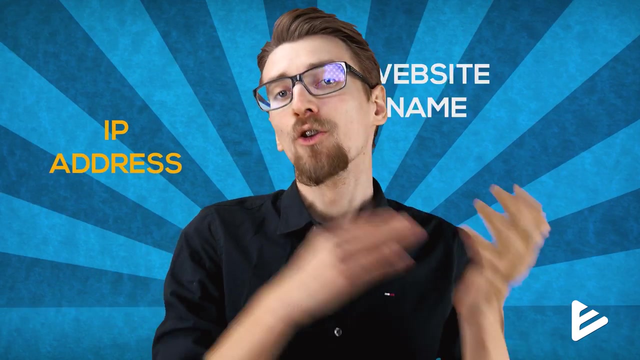 files on your computer that allows incoming connections. That means it basically mimics a web hosting server. Problem is, people can only connect to your website using an IP address, and IP addresses are not easy to remember, So next I'll show you how to connect the website name to the IP address so they 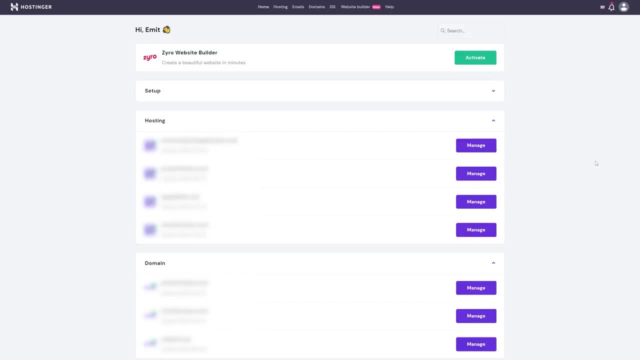 can use that instead To link your domain name to the IP address. you just have to change some DNS settings. So I'm going to use Hostinger for this. Go to your dashboard and click manage. near your domain name, Find the DNS zone tab. 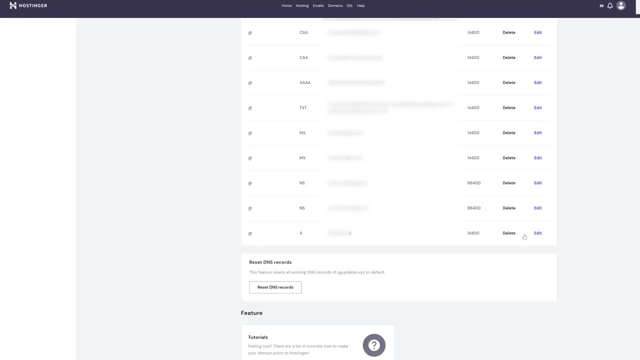 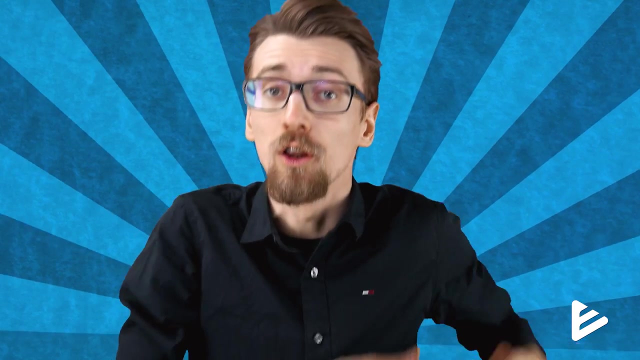 and click on edit, You'll need to edit your a host record Here. type in your IP address instead of the one that's here. This way, your website name will link to your IP address. Okay, so what we did is we basically created a website that's hosted locally but can be accessed by a specific IP. 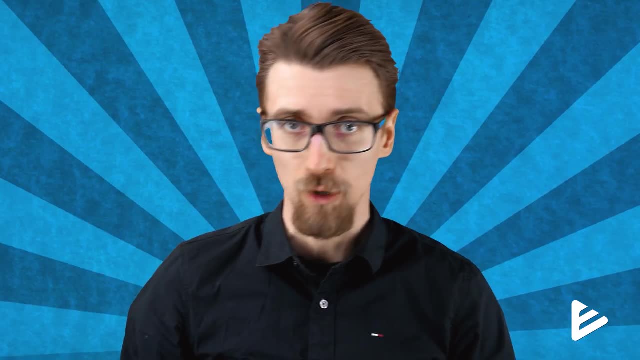 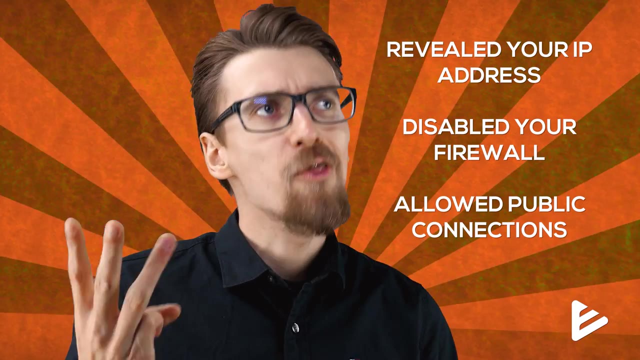 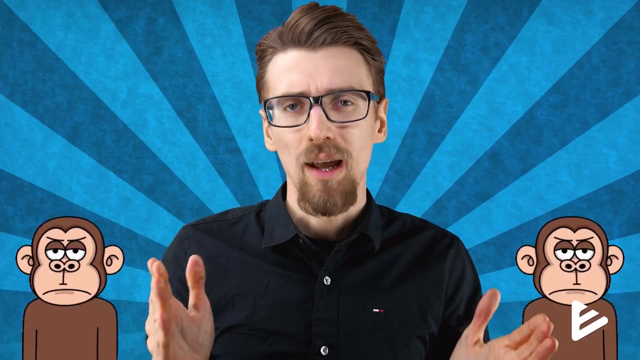 address or a domain name pointed to that IP address, Or in other words, you just revealed your IP address to the whole world, You disabled your firewall and then you allowed incoming connections to your computer without any security. Yeah, it's, it's that dumb and a huge security risk. So please do not do this. Get cheap.